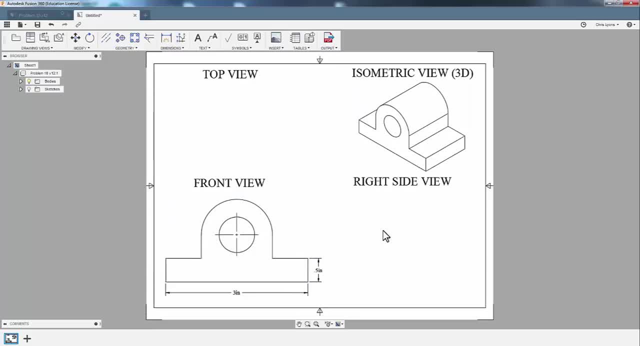 we're going to represent with a series of two-dimensional drawings, and the reason we're going to do that is so that we can clearly see all details. In the lower left hand corner of an orthographic drawing, you'll always be able to see the front view. That is the most important view. 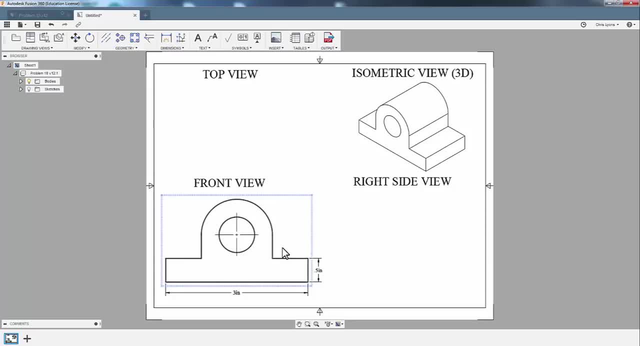 and the one that each other view is based off of, Directly above or on top of the front view. you will always see the top view And you'll notice that when you draw these or create them, that it should stay aligned with the front view. So you can see that they are staying aligned. I can't move this side to side. They. 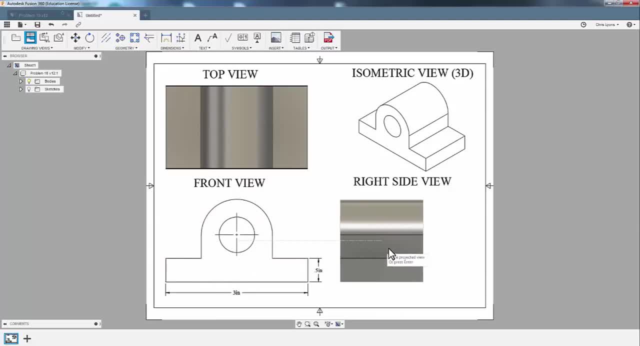 should be lined up, And the reason that they should be lined up with the front view is so that it's easier to understand all the details and label the drawing with measurements. Now, as we're looking at each view, there are a couple things that we need to understand. Notice: they share the same base. 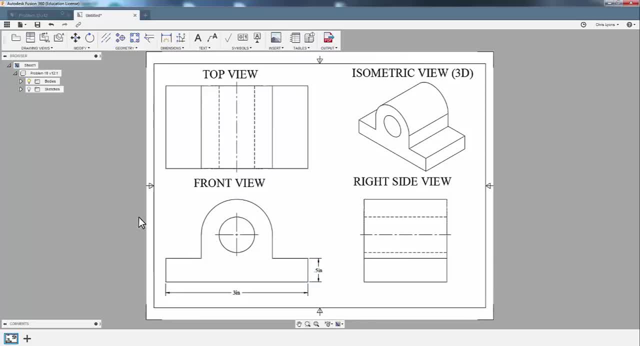 All the measurements are the same. Each view is drawn to the same size. In the engineering world we refer to that as the same scale. Scale is the size of the drawing in relation to real life. I can see down here that the width or length of the item is three inches. 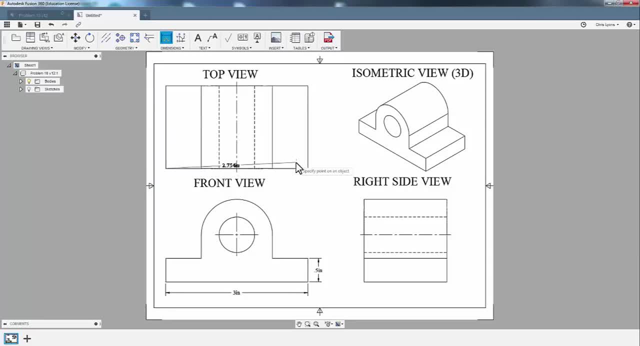 If I were to measure that in the top view, I would notice that it's also three inches, So the size proportions are the same. So why might we want to have three different views of an object? Because we might be able to see details in. 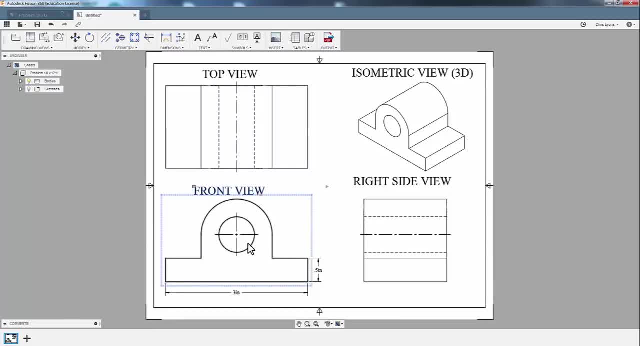 opposite views that we can't in others. So, for example, the front view. I can see there's a circle here, a hole, but I don't know how deep it is. In the top view I can see that it does go all the way through the object. 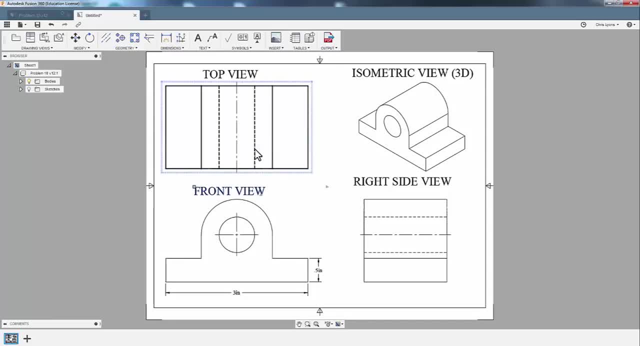 That is represented by these dashed lines. here and here, Those dashed lines represent hidden lines, A line that exists but cannot be seen from up above. I still need to know it's there. so, instead of a solid line which represents boundaries, where an object ends or a corner, 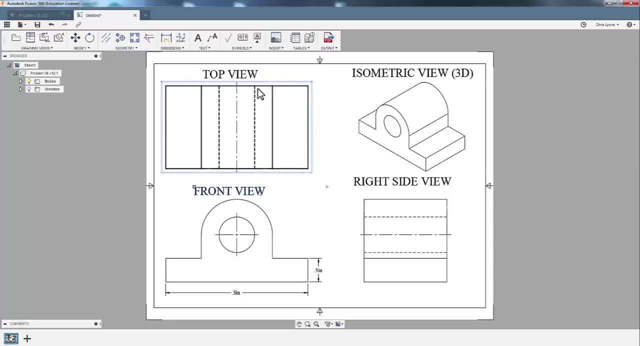 exists. I draw those as dashed lines: A spot where a line exists, an edge, but cannot be seen. I can also see that over here, in the right side view, And if I drew a line, I would notice that the top of the hole lines up with the dashed lines over here. 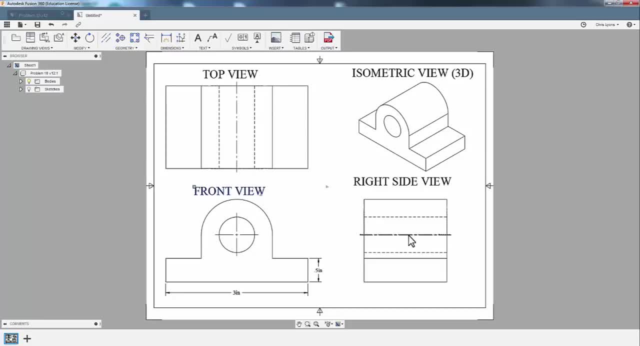 Now, in between those you'll see a long dash and short dashed line That represents the center of that hole. Here in the front view you'll notice you have a center mark, a plus, so to speak, That marks the center point of the hole. 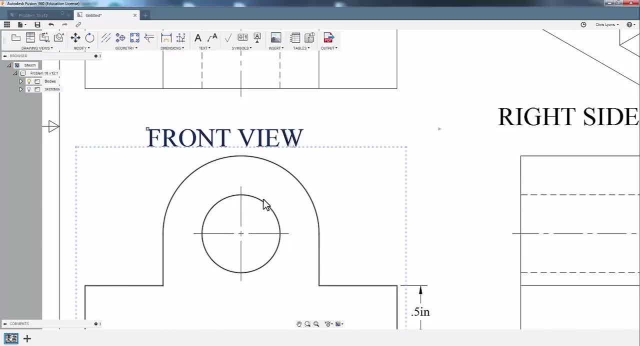 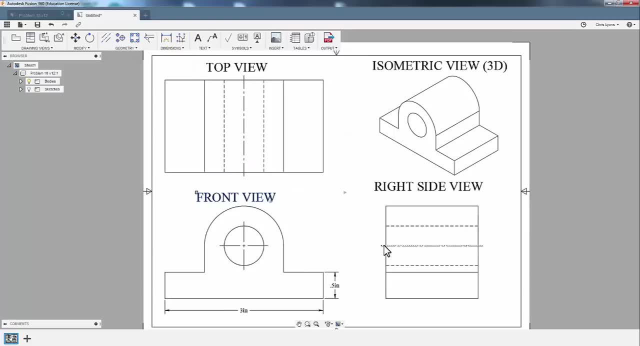 And they're also measured from the center to narrate their size. We also want to label that center line in views where it can't be seen as a circle or a hole, so that you understand that it is some type of circle or arc or curve. 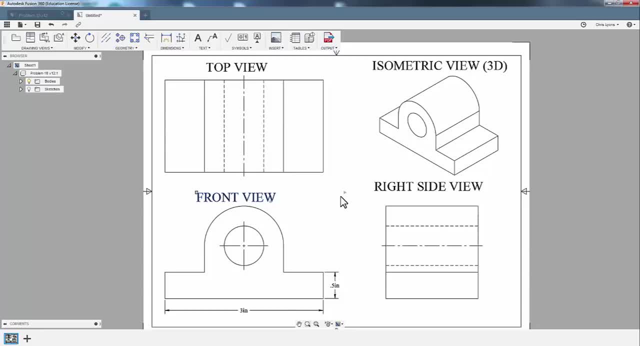 And it makes it easier to see and understand those details. When you're reading these, you are going to need to understand how to look at the size dimensions. So here I can see the depth is 1.75.. If I look at the right side view, I can also see that it is labeled 1.75.. 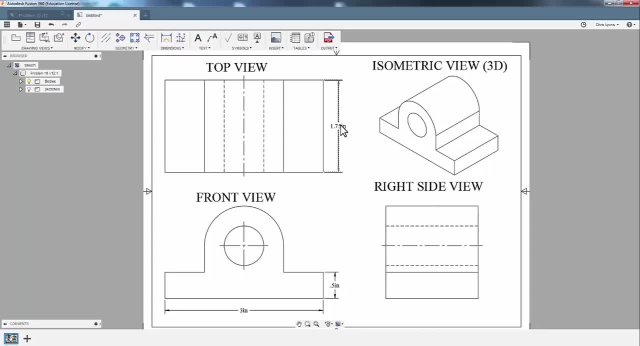 If a dimension is only labeled in one spot, it doesn't mean that this is different. They are the same. Those dimensions are the same, and to label it more than one time would be redundant. You wouldn't want to do that, So, off of these drawings, you're going to need to be able to get a couple of different measurements. 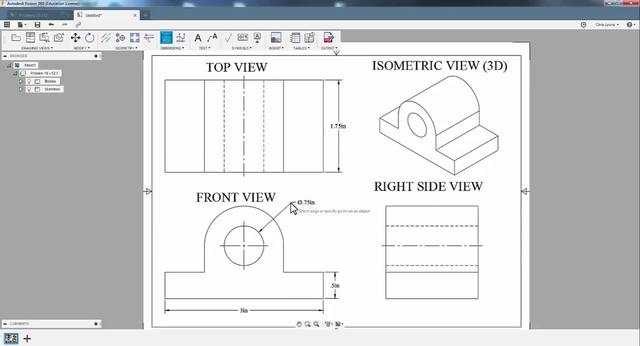 Here. we need to know the diameter of that hole, We're going to want to know the radius of the arc, And you're going to need to know various heights and widths of parts of the object. on the screen, I should be able to look at the front view and gather most of the details I need. 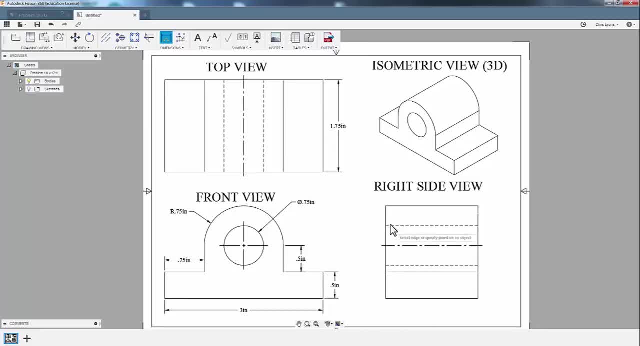 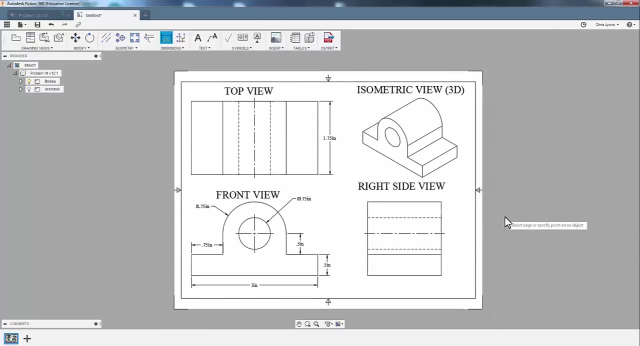 Any details that might be missing can be located in the right side view Or the top view. Take a look at the fusion problems that you're going to create in 3D modeling on the next page on Schoology And start to analyze how those pieces are put on the screen. 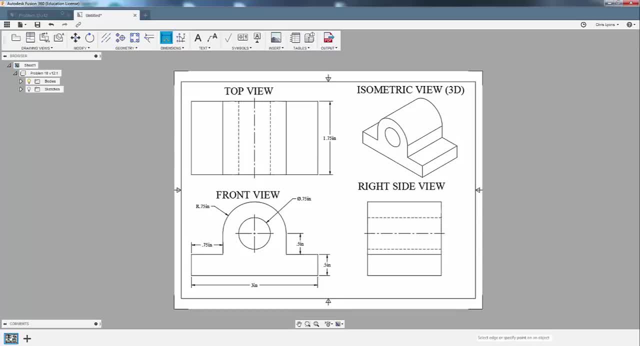 And try to solve for the measurements.